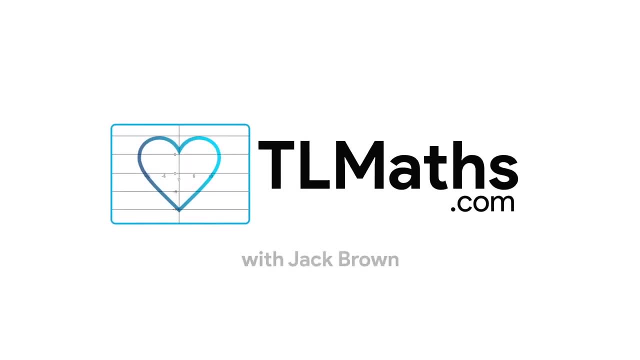 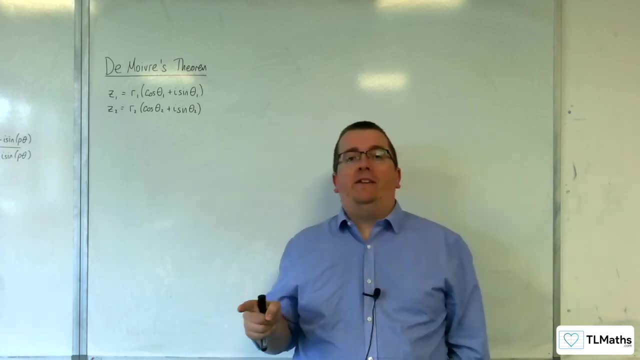 So in this video I'd like to introduce you to de Moivre's theorem, which actually I've proved already back in the proof by induction section. It's quite a good proof by induction to do So. I'm going to introduce you to where the idea is going to come from. I'm not going 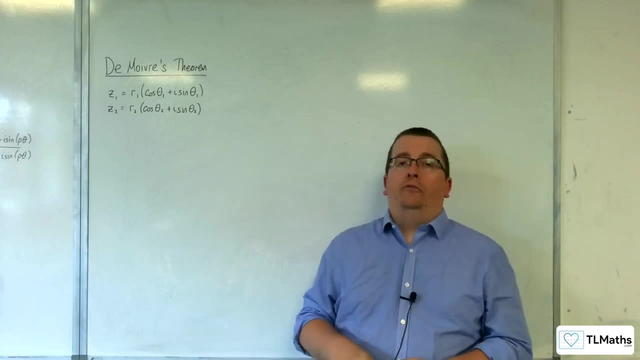 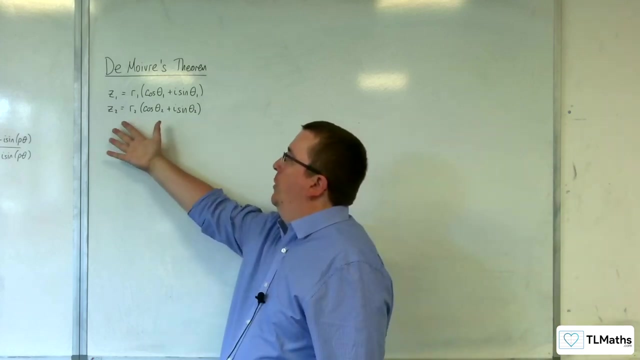 to prove it again. You can go back and see that proof in section A, But that proof only worked for positive integer values of n and I'm going to prove it for negative integer values of n. So let's rewind and let's go back to thinking about if I've got two complex 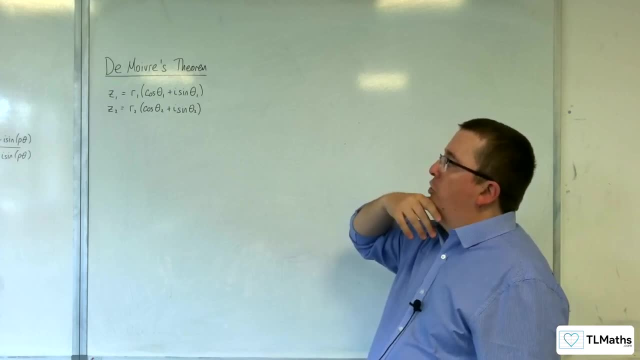 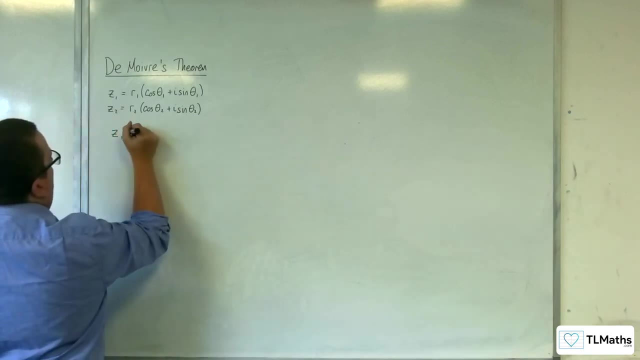 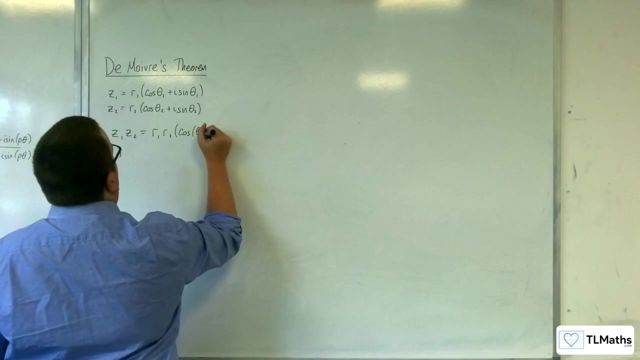 numbers, so z1 and z2, and I've written them in modulus argument form. We saw that if you multiplied z1 by z2, that would be the same as multiplying the two modulus okay, r1, r2, and you add the arguments, So you get cosine of theta1 plus theta2 plus. 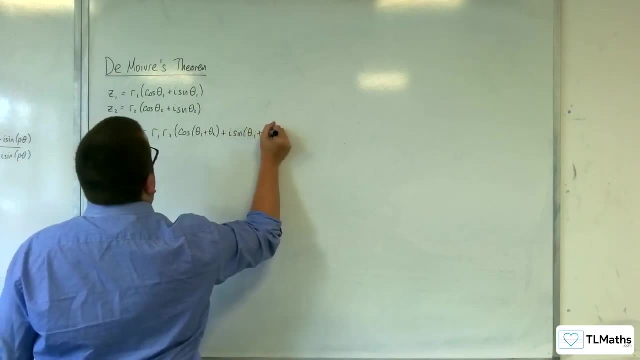 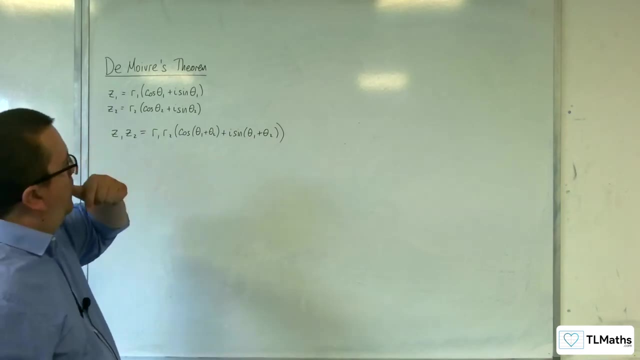 i sine of theta1 plus theta2.. Okay, so that's what we have done. That's what we've already seen in this section. Now, if we'd actually done z1 times z1, so z1 squared okay, then the idea would then be that, having done z1 times z1, I would have 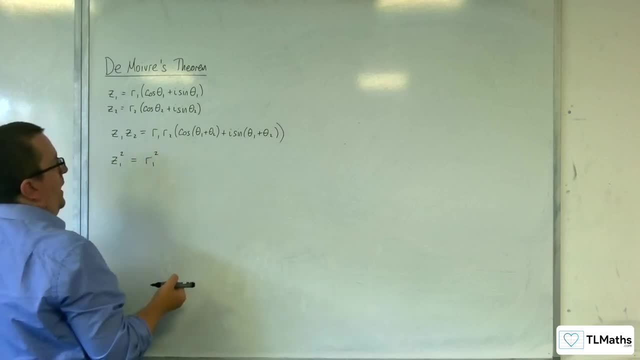 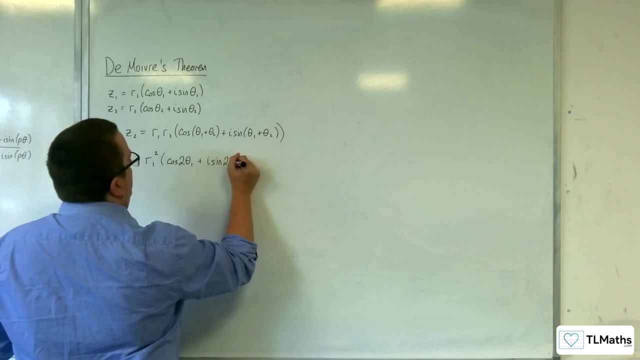 r1 times r1,, which would be r1 squared, and you'd have cosine of theta1 plus theta1,, which is cosine of 2 theta1,, and you'd have theta1 plus theta1 here. so i sine of 2 theta1, okay. 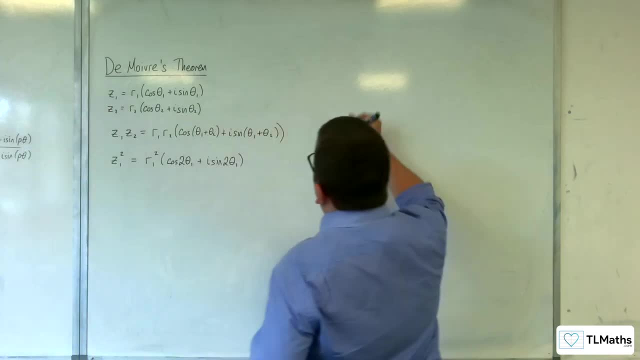 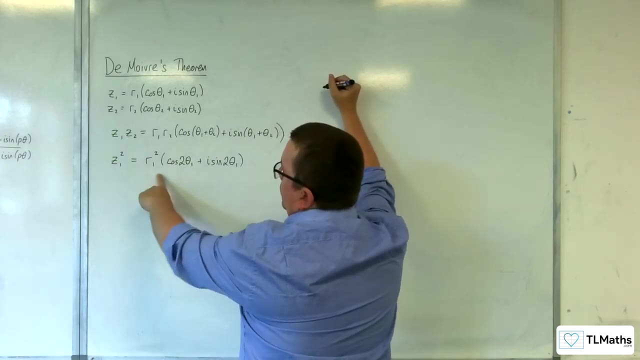 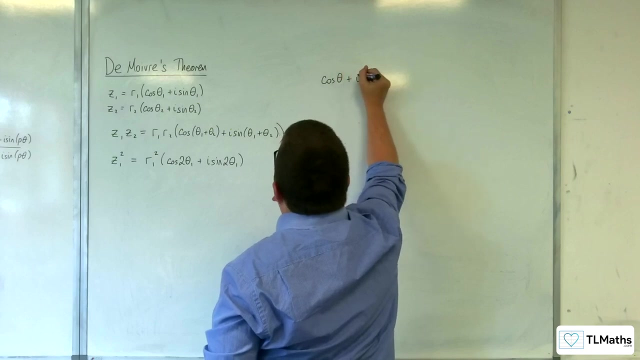 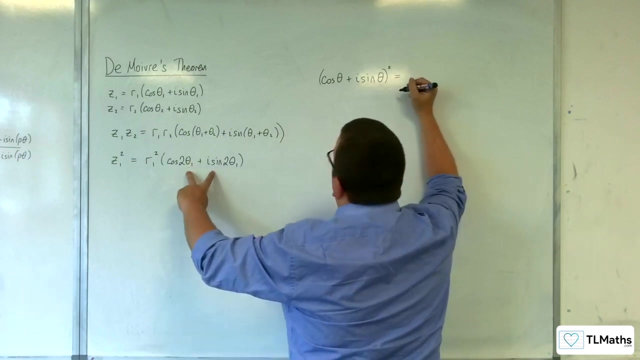 So what this is showing is that if you've got now- I'll ignore the r for the time being- okay. So let's just imagine that r is 1, okay, If you've got cosine of theta plus i sine of theta and you square it, then what you get is this: You get cosine of 2 theta. 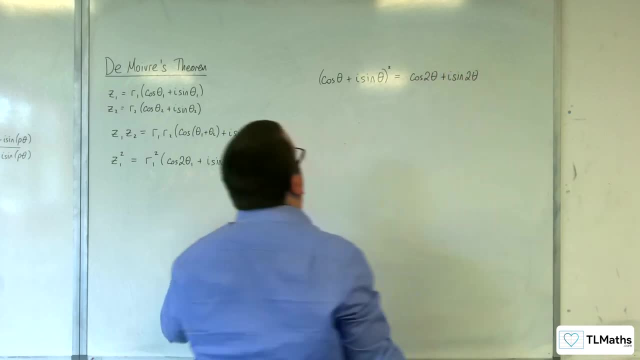 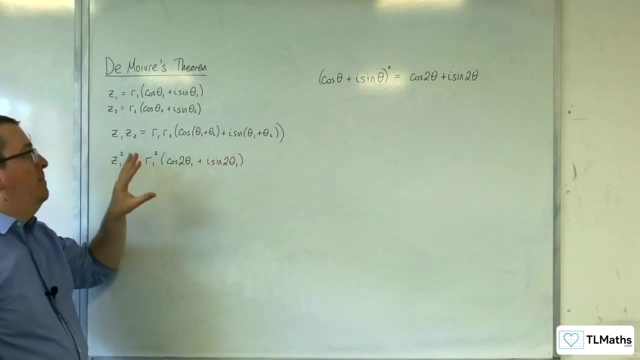 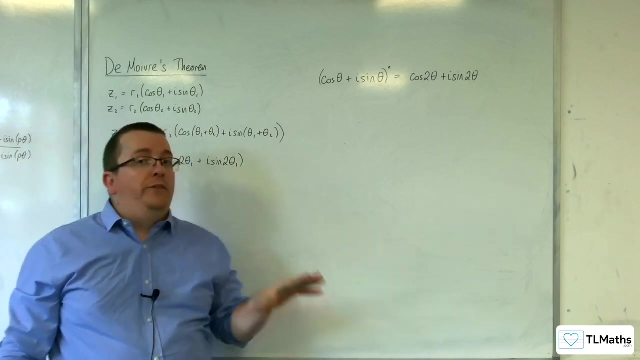 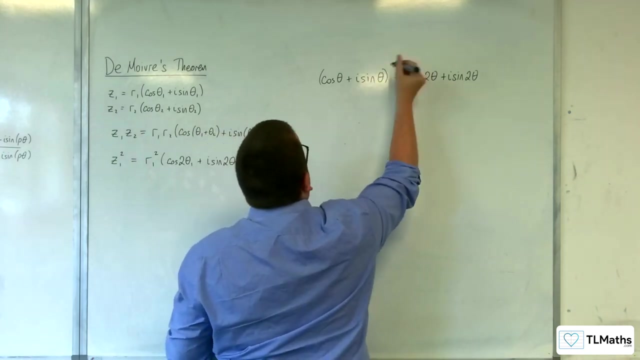 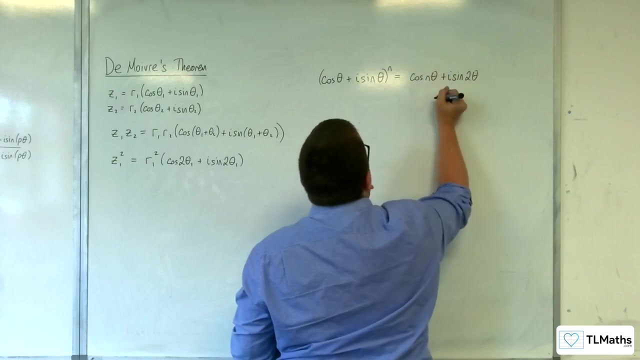 plus i sine 2 theta. okay, So that is a direct result from what we've seen by multiplying complex numbers together when they're in modulus argument form. Now DeMoyer's theorem goes one step further. Okay. Moira's theorem says that actually if you have cosine theta plus i sine theta to the n, then cosine that is cosine of n theta plus i sine of n theta. 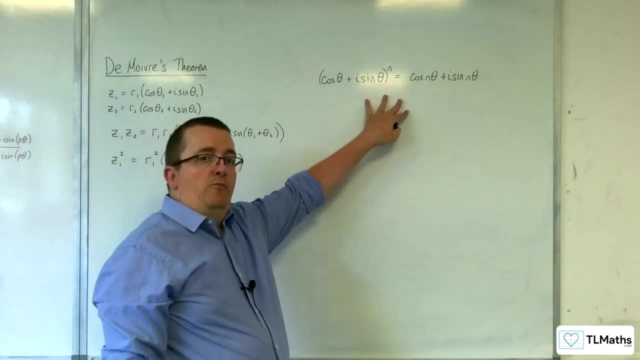 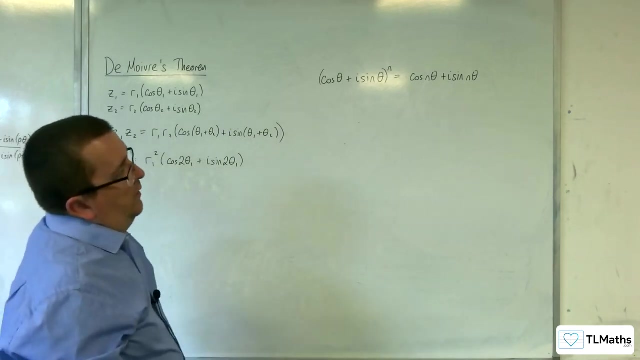 Okay, and I've proved that for all positive values of n, positive integer values of n- okay, using proof by induction. So that's proved back in section a: okay, So it would be nice if we could also work with negative values of n. okay, and that's what I'm going to prove here. 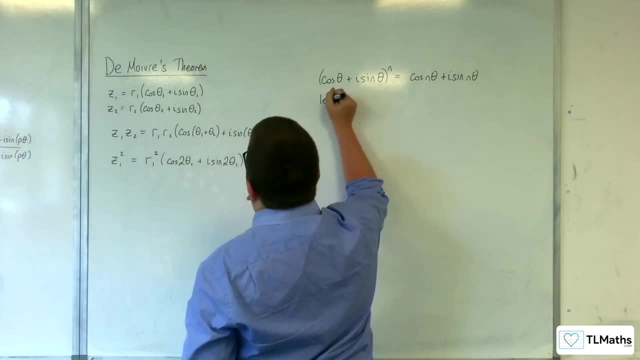 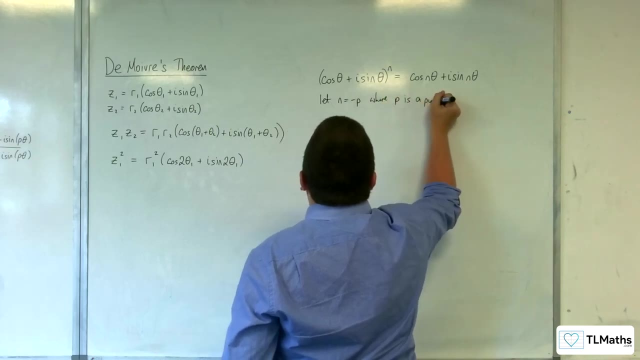 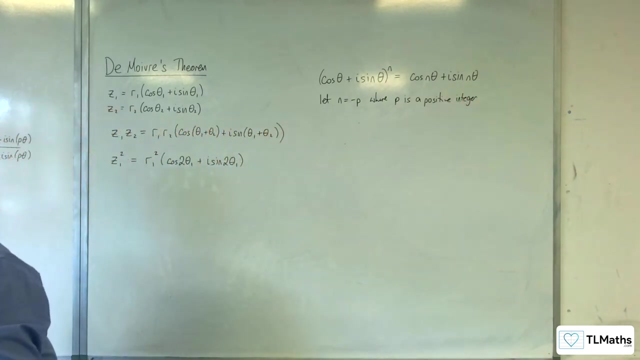 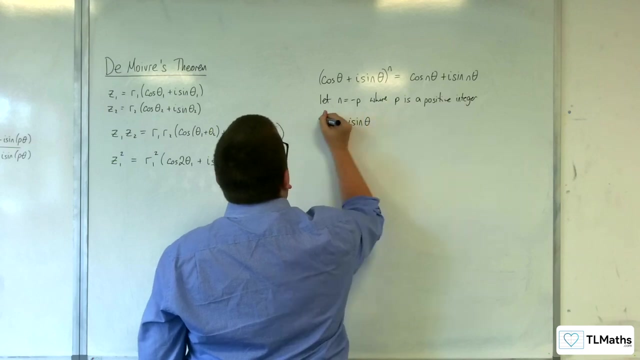 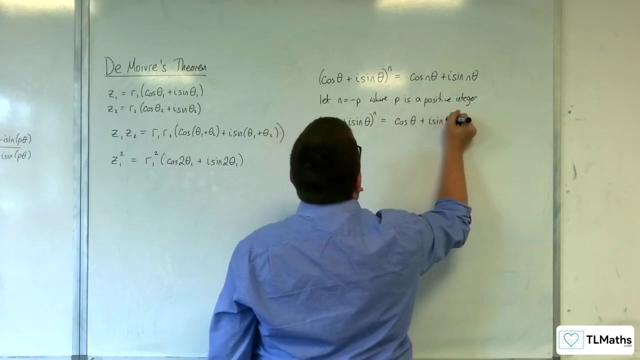 So let's say that let n equal minus p where p is a positive integer. okay. So that would mean that we would have cosine theta plus i sine theta to the n is now cosine theta plus i sine theta to the minus p, okay. 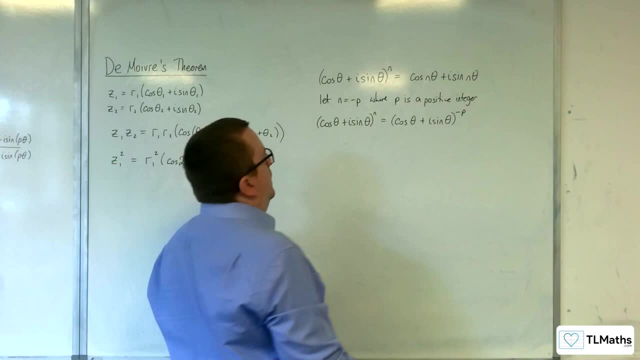 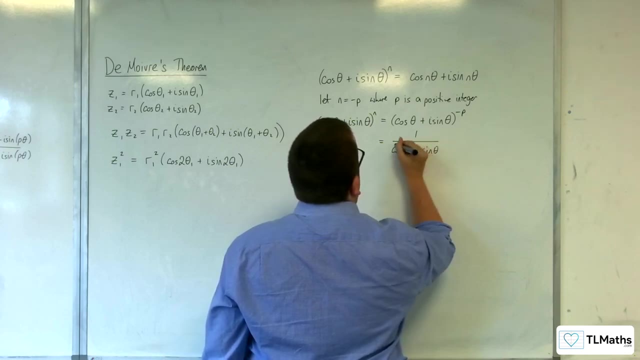 So I've replaced the n with minus p. Now that is the same as 1 over cosine theta plus i sine theta To the p. okay, But remember, p is a positive integer and I've proved this for positive values. positive integer values of n. 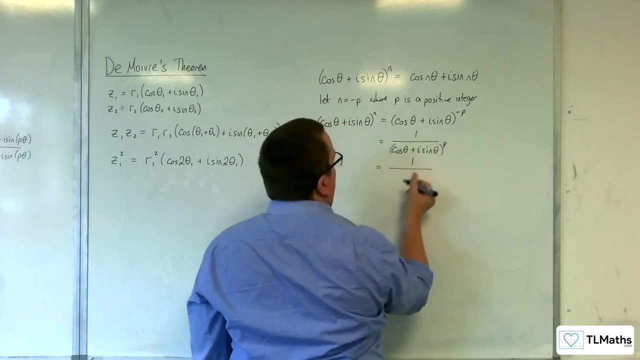 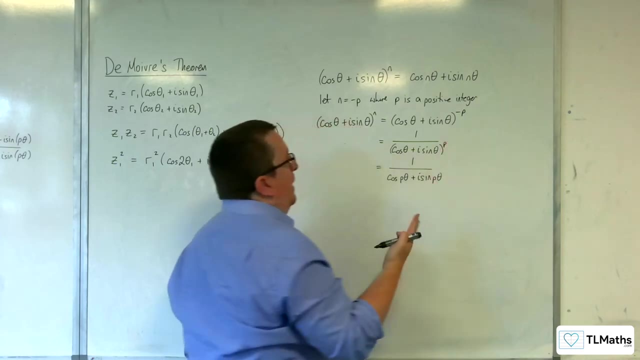 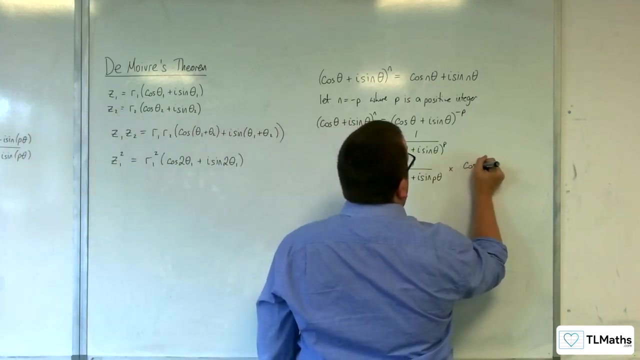 So that means I'm perfectly at liberty to bring that p down and write that as cosine of p theta plus i sine of p theta, Because here p- remember- is a positive integer. So that's perfectly valid. Now, if you multiply this top and bottom, 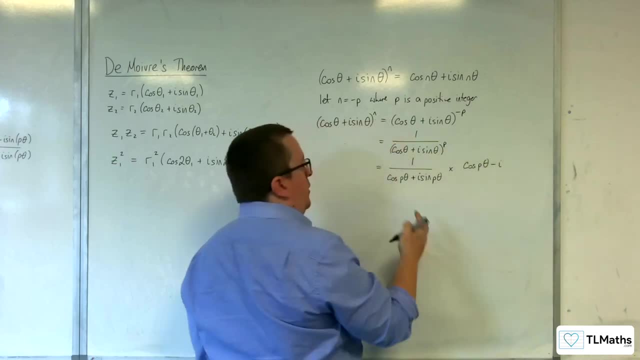 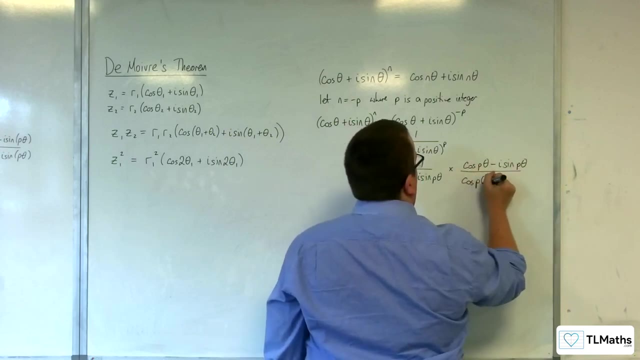 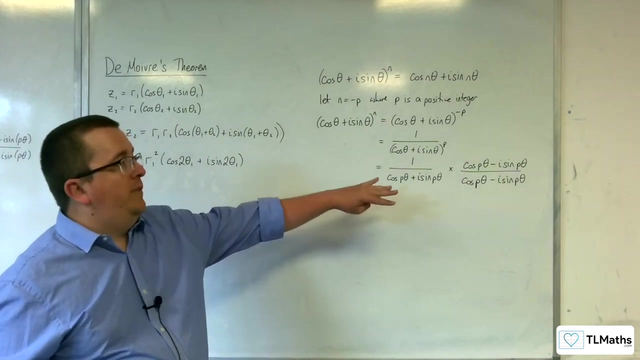 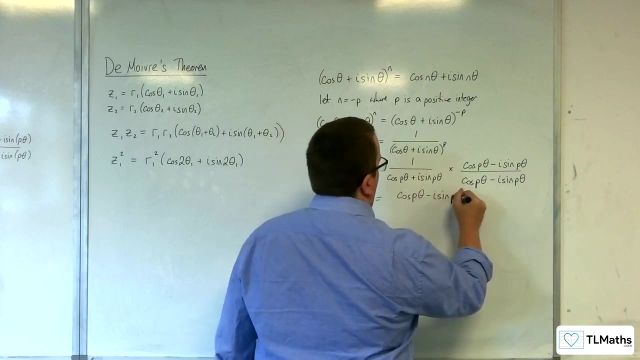 So, just as we would have done by multiplying top and bottom by the complex conjugate of the denominator Like: so okay, Well, your numerator is just going to be cosine p- theta. take away i sine of p- theta. Okay, Okay, In the denominator you're going to get cosine p theta times cosine p. 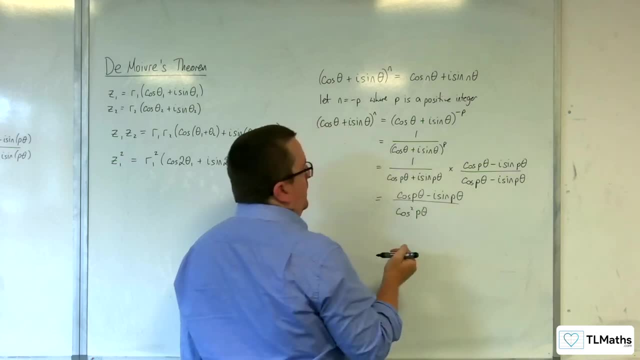 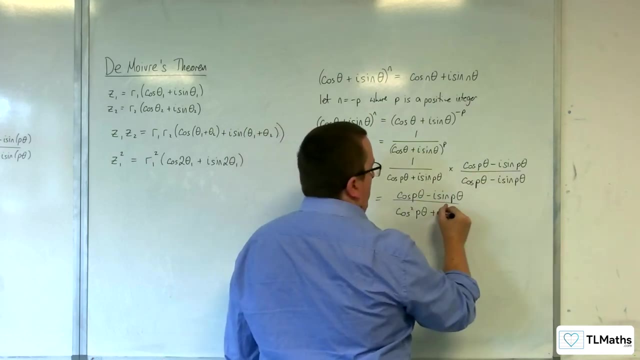 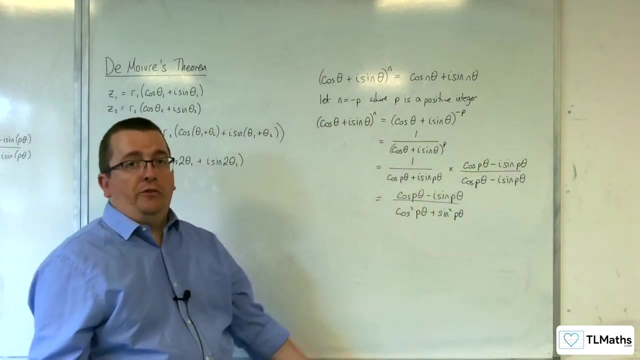 So cosine squared of p theta, The middle terms are going to cancel And you're going to get the i sine p theta times minus i sine p theta, which is plus sine squared p theta. So in the denominator you've got sine squared plus cosine squared, which of course is 1.. 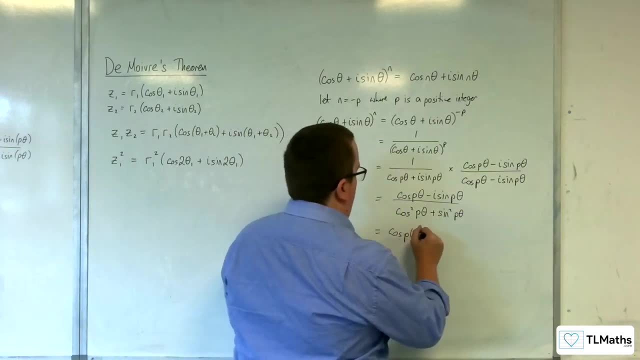 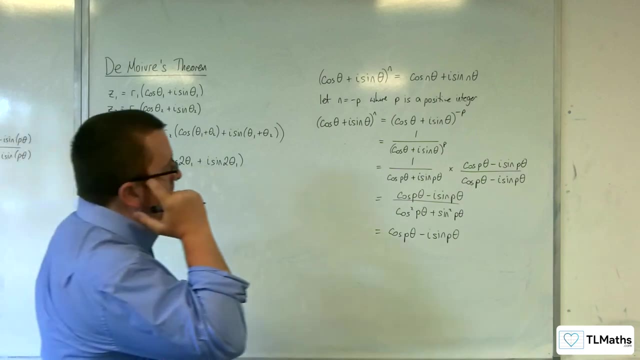 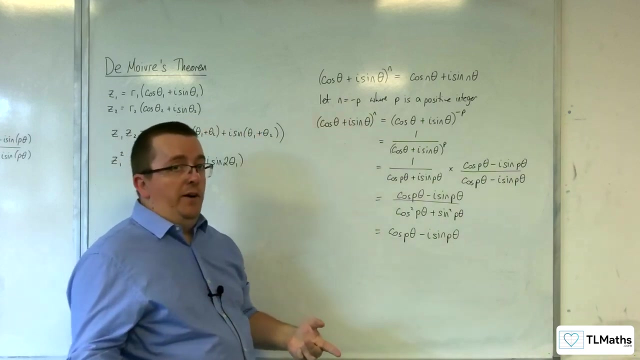 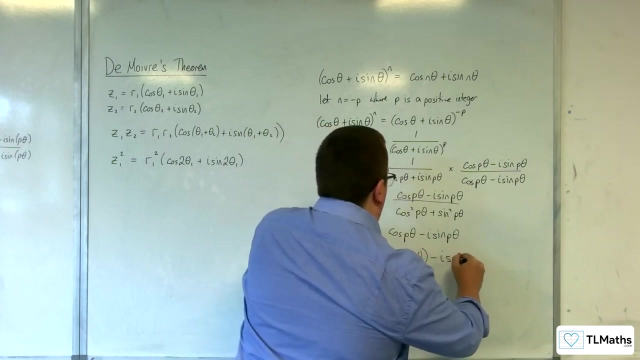 So this is cosine of p theta. take away i sine of p theta. Okay, Now remember n was equal to minus p, So p is equal to minus n. So if I swap back in, I'm now at minus n theta. take away i sine of minus n theta. 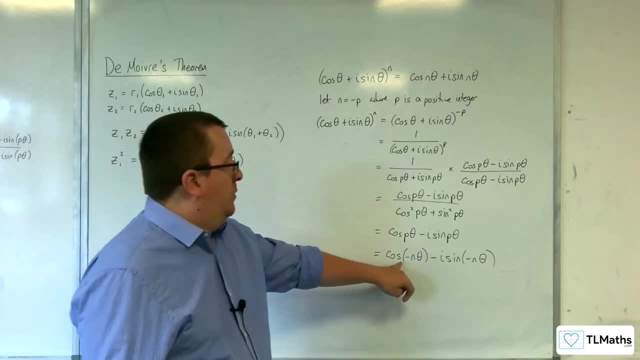 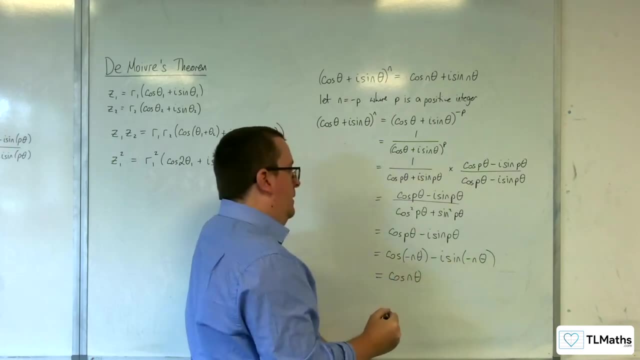 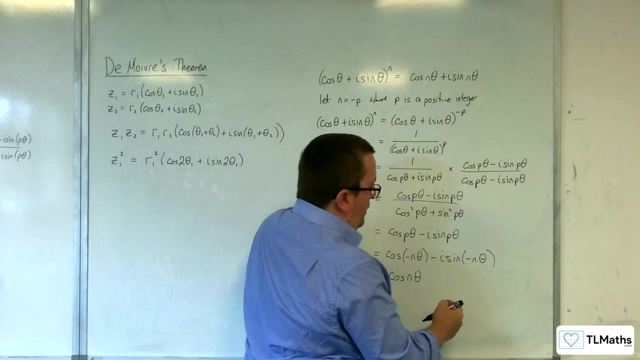 But cosine is an even function, So cosine of minus n theta is the same thing as cosine of n theta, And sine is an odd function. Okay, So that minus sine can come out and multiply with that minus sine And you'll get plus i sine of n theta. 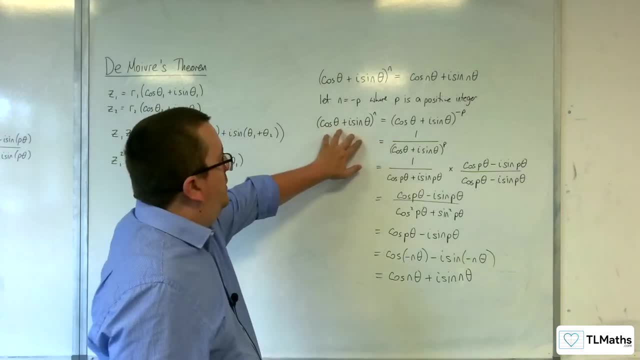 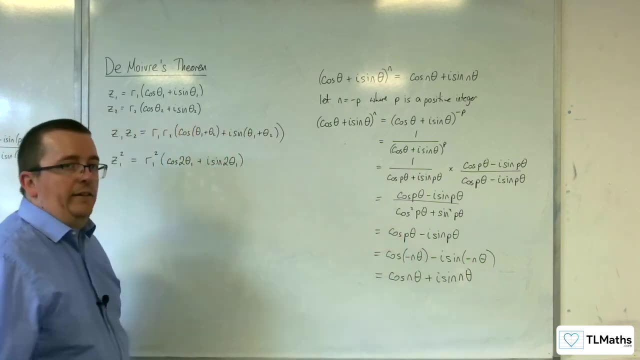 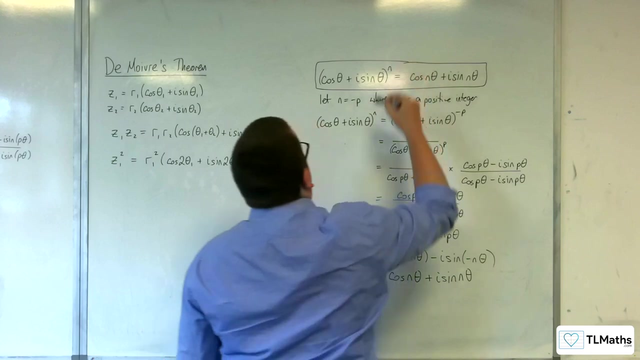 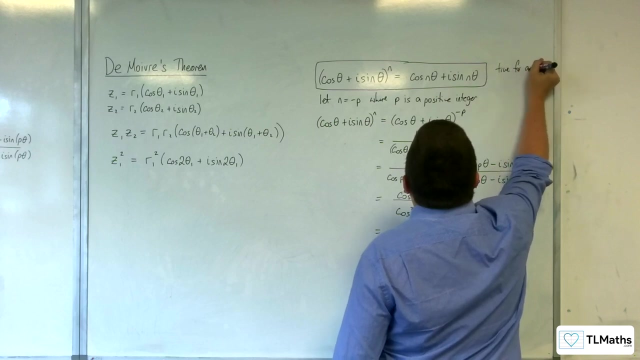 And so cosine of theta plus i sine of theta to the n is the same as cosine of n theta plus i sine of n theta, where n is a negative integer, And so the Moivre's theorem here is true for all integers n Okay. 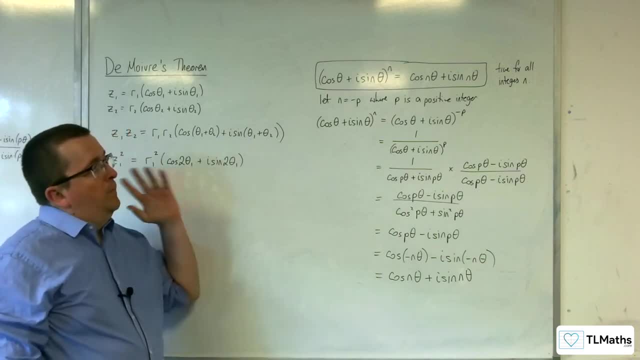 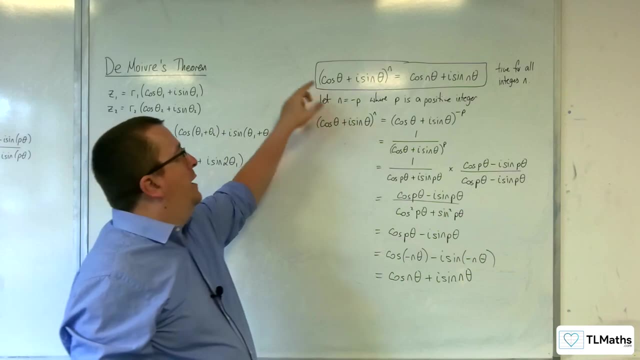 So, with that then in mind, okay, we now have a theorem that will allow us to simplify things A great deal. Okay, And we're going to be working with the Moivre's theorem in this set of videos.